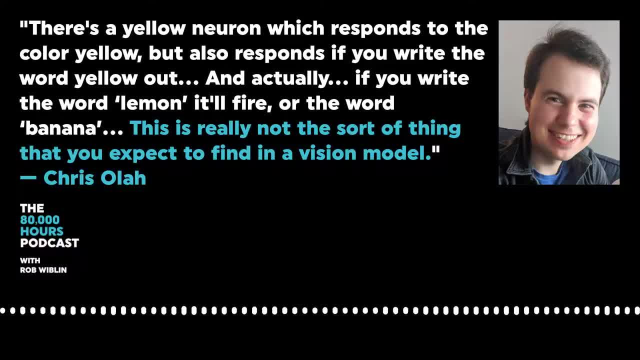 So we were investigating this model called CLIP from OpenAI, which you can roughly think of as being trained to caption images or to pair images with their captions. So it's not classifying images, It's doing something a little bit different, And we found a lot of things that 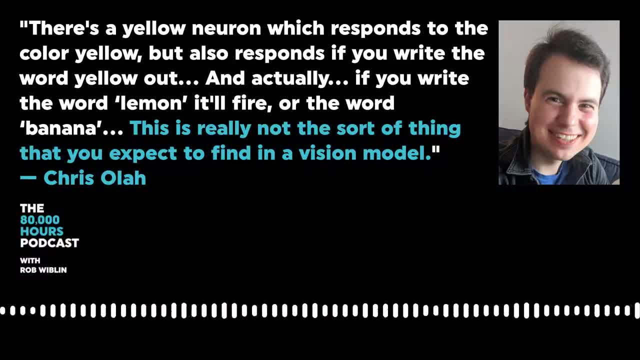 were really deeply qualitatively different inside it. So if you look at low-level vision, actually a lot of it is very similar And again it's actually further evidence for universality. A lot of the same things we find in other vision models occur also in early vision in CLIP. 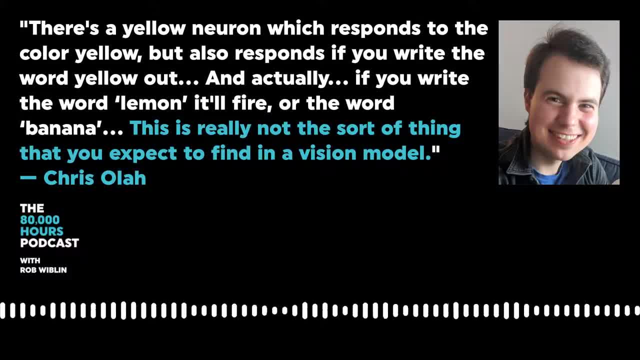 But towards the end we find these incredibly abstract neurons that are just very different from anything we'd seen before. And one thing that's really interesting about these neurons is they can read, They can go and recognize text and images and they fuse this together. 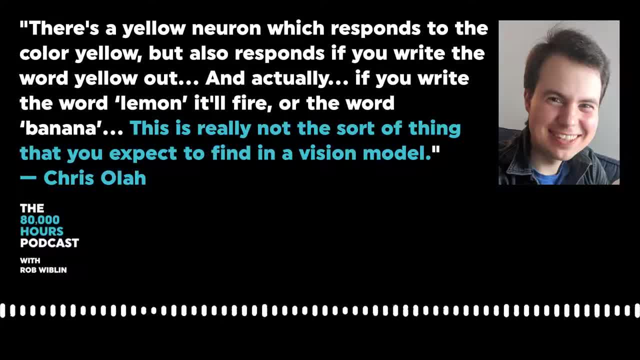 So they fuse it together with the thing that's being detected. So there's a yellow neuron, for instance, which responds to the color yellow. but it also responds if you write the word yellow out and it will fire as well. And actually it'll fire if you write out the word yellow. 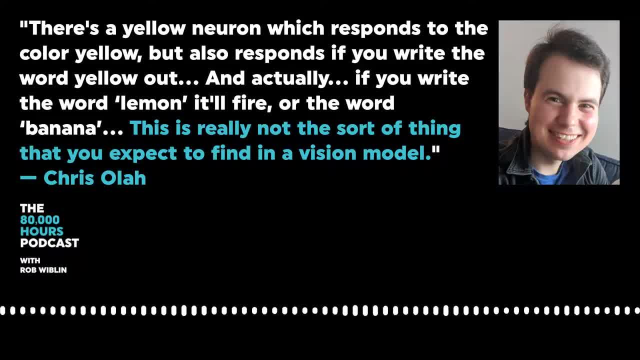 words for objects that are yellow. So if you write the word lemon, it'll fire, or the word banana, it'll fire, And this is really not the sort of thing that you expect to find in a vision model. It's, in some sense it's a vision model, but it's almost doing linguistic processing in. 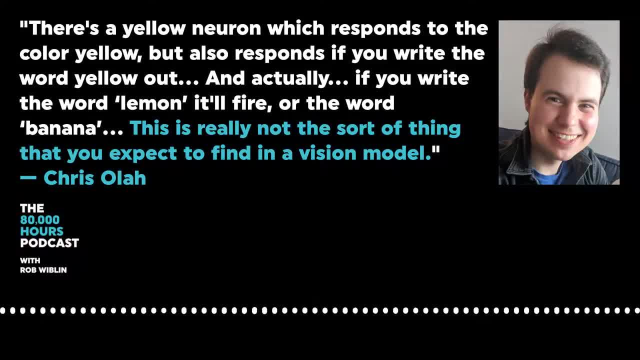 some way And it's fusing it together into what we call these multimodal neurons, And this is a phenomenon that has been found in neuroscience. So you find these neurons also for people Like there's a Spider-Man neuron that fires both for the word Spider-Man. 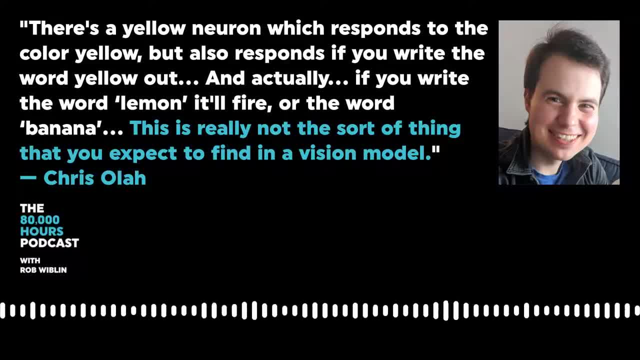 as an image, like a picture of the word Spider-Man and also for pictures of Spider-Man and for drawings of Spider-Man. And this mirror is a really famous result from neuroscience of the Haley-Berry neuron or the Jennifer Aniston neuron, which also respond to pictures of the 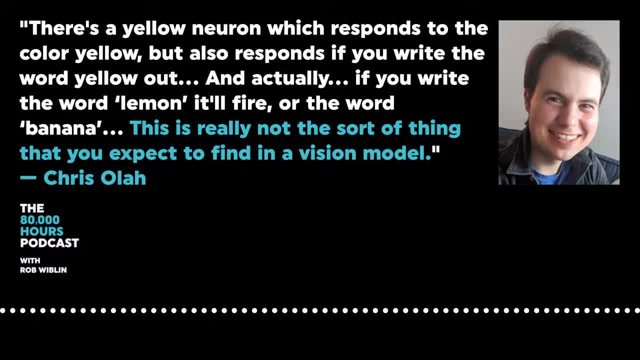 person and to drawings of the person and to the person's name, And so these neurons seem in some sense much more abstract and almost conceptual compared to the previous neurons that we found, And they span an incredible wide range of topics. In fact, a lot of the neurons-